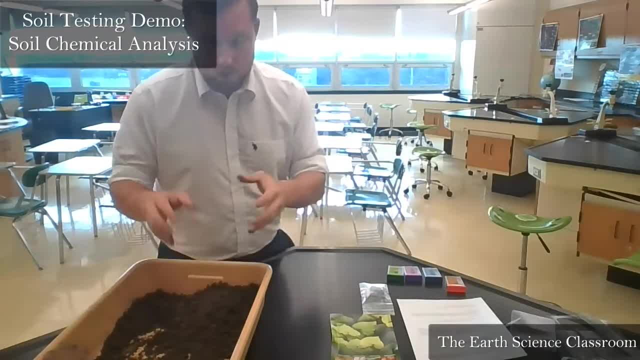 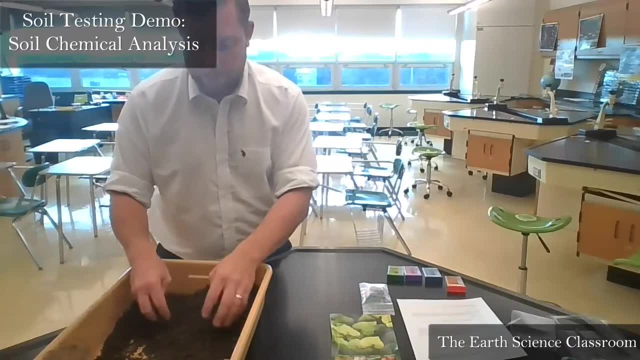 and we have no more life on the planet. The soil is a big deal Now. the chemical analysis involves four things. looking at pH Now. pH is the measure of the amount of hydrogen ions in the soil. Basically, it means that if there is a high amount, it will be acidic. 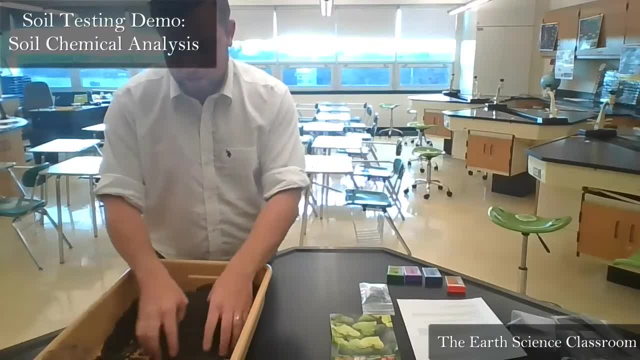 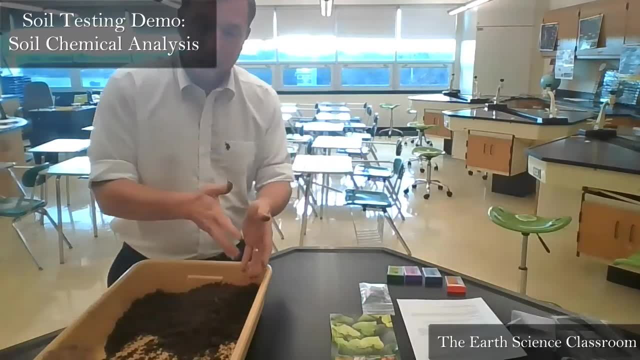 If there's a low amount it will be a base or alkali, And certain plants like to have more of an acidic soil, so it's more hydrogen ions, and some plants like to have more alkali or base soils. So we test the soil to see what kind of plants would like to grow in. 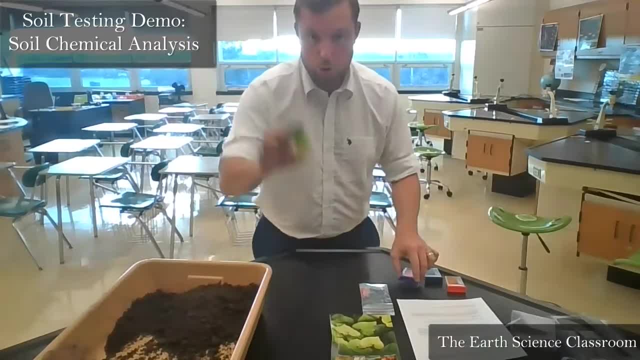 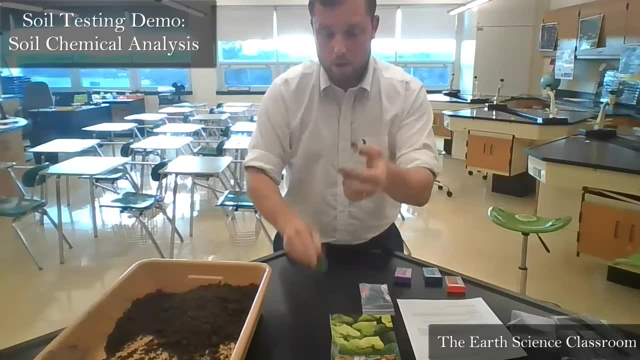 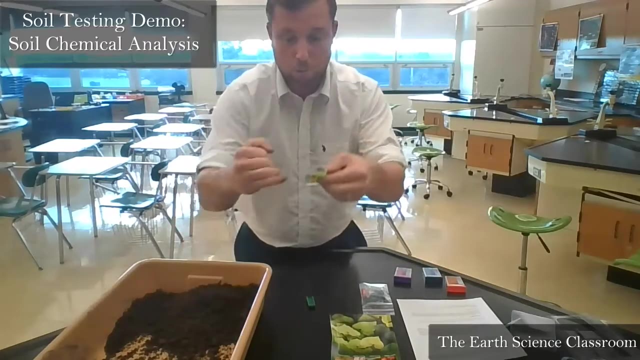 this soil. So we have our little tubes right here, our little equipment, and it's very simple. You take the cap off, alright, like so, and you have this small area and the large area. you always put the soil into the small area, you get a little little pinch of. 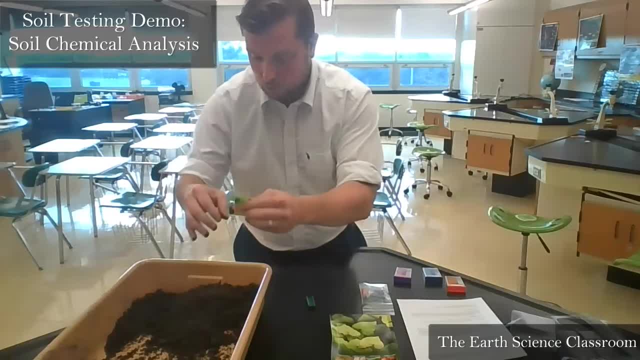 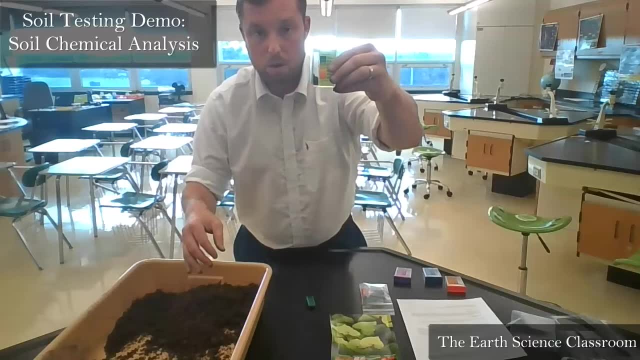 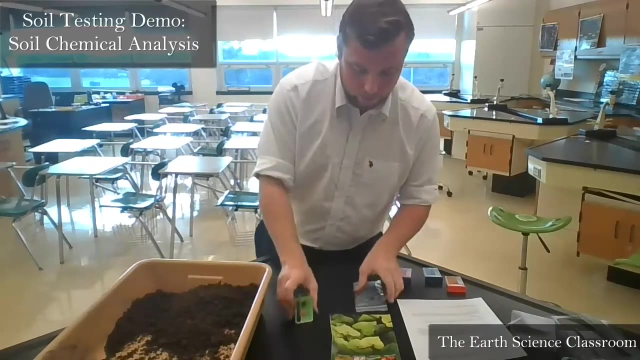 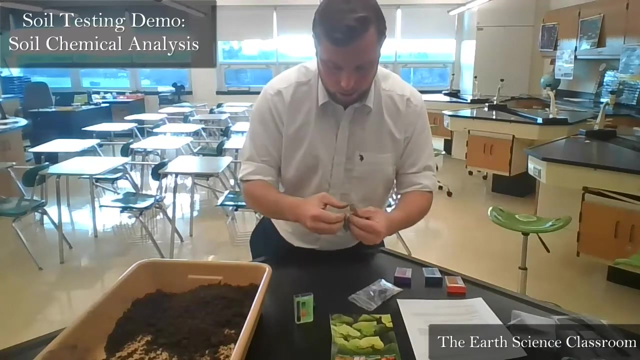 soil with our fingertips and we put in a little bit of soil, a little bit of soil in the bottom, like so, okay, a little bit of soil, just right there. then we have working with ph right now. so it's the green capsule. so you correspond the green capsule with your green chemical indicator. 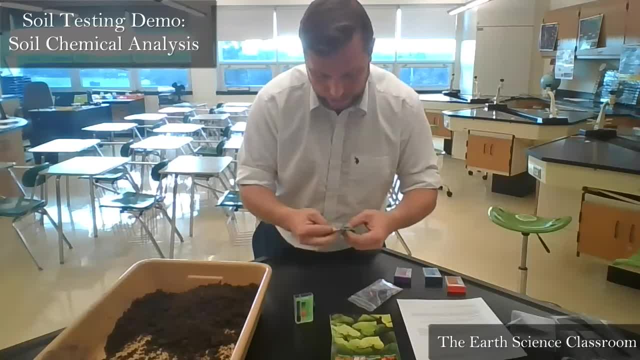 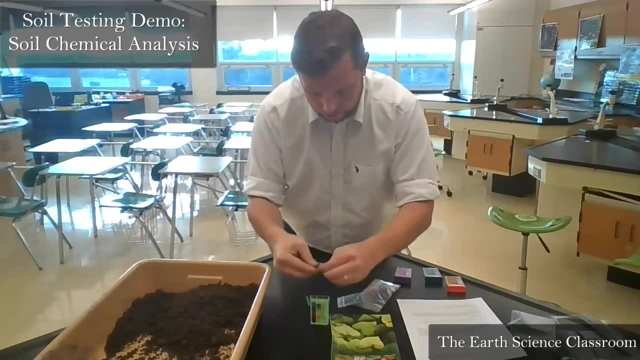 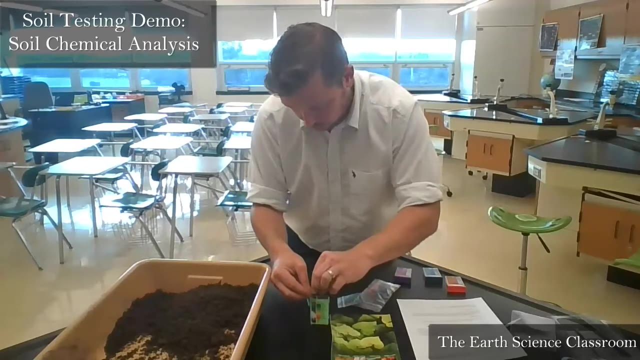 you put this stuff in a little capsule and you twist it to the left or to the right with both hands. you twist it and you pour the contents into on top of the soil. so first goes soil, then you pour the contents into the soil, and then you pour the contents into the soil. 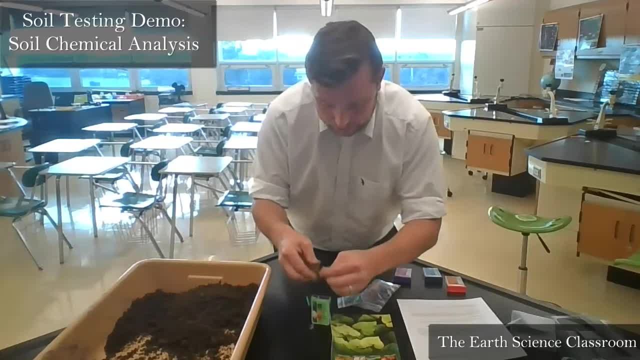 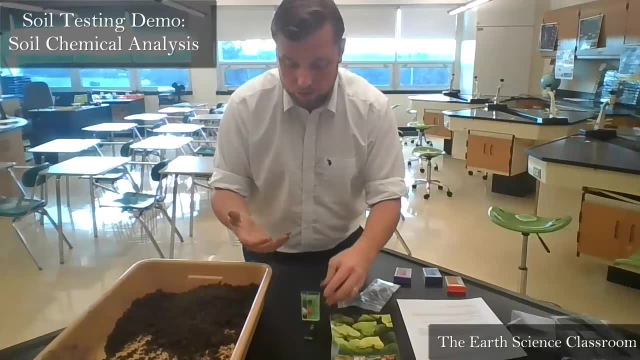 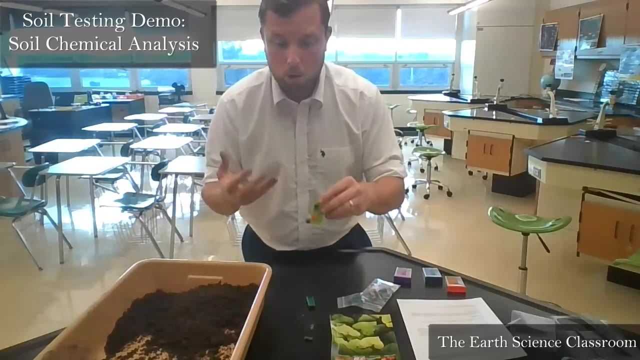 then goes the chemicals. okay, this is a chemical indicator. just as lab safety goes on your hands- please wash your hands thoroughly- goes on your skin- please wash your skin. do not eat this stuff. it is not sugar. we don't eat anything that we work with in a lab. okay, just as a general. 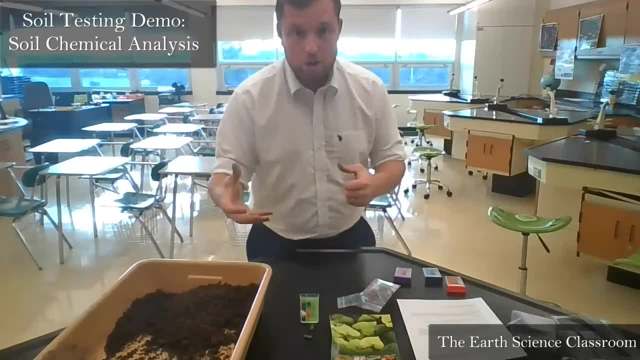 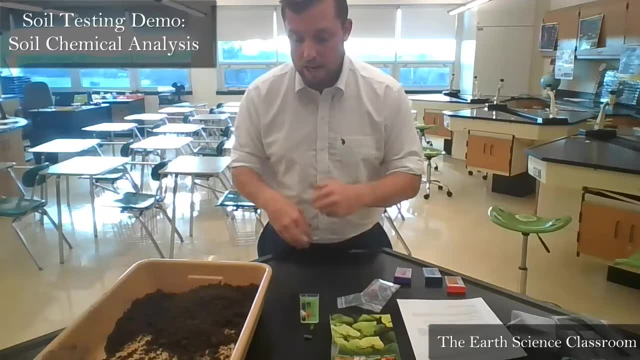 precaution general guideline: we don't eat anything. if you go into lunch after this period, you want make sure you go to the bathroom and you wash your hands thoroughly with water and soap, okay, so please don't eat with any chemicals on your hands now. if you want to use gloves, we have gloves. 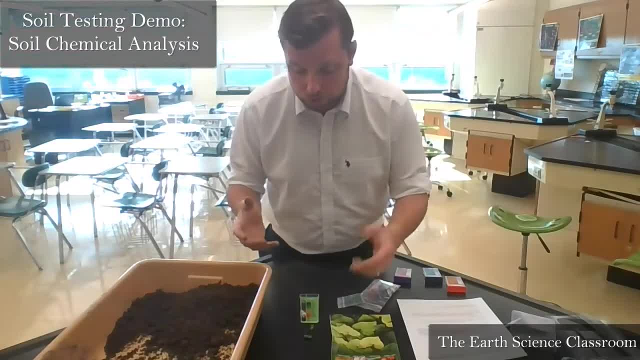 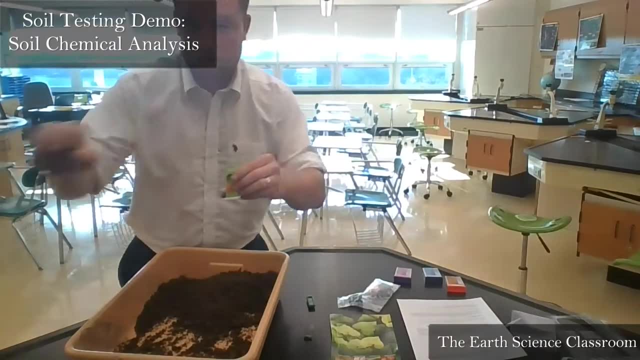 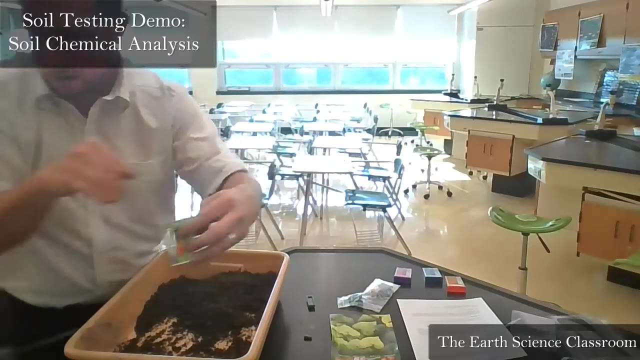 in the corner, um, so feel free to use gloves if you want to. now you take this. you have the soil and the chemical indicator. you add some water, but very small amount of water. okay, i'm going to fill water up this little dash line at the top here. that's the point where you add water. so it's a. 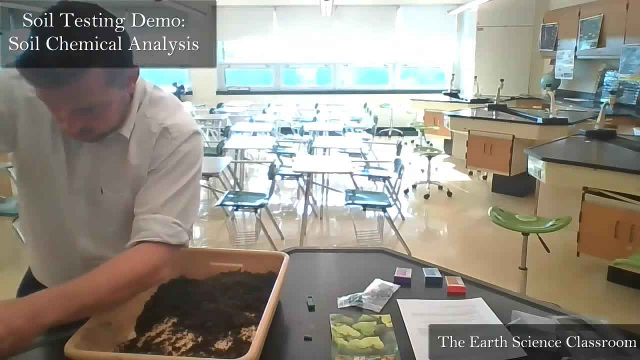 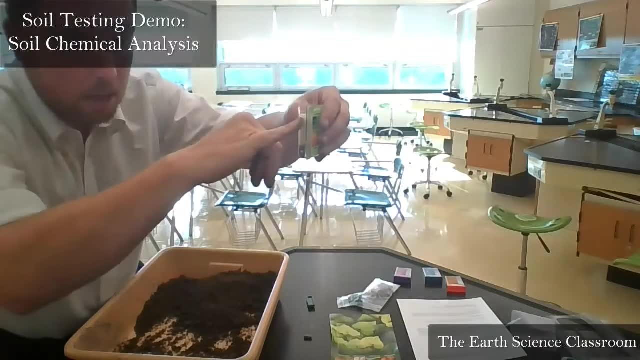 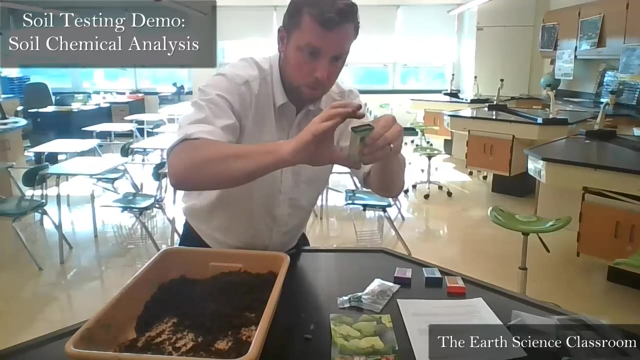 small amount of water, a little trickle of water like that. okay, so we've got the water here, soil and the chemical. now again we put back the lid on top. make sure the lid's on properly. we have. we hold it like this: thumb and forefinger we hold it. 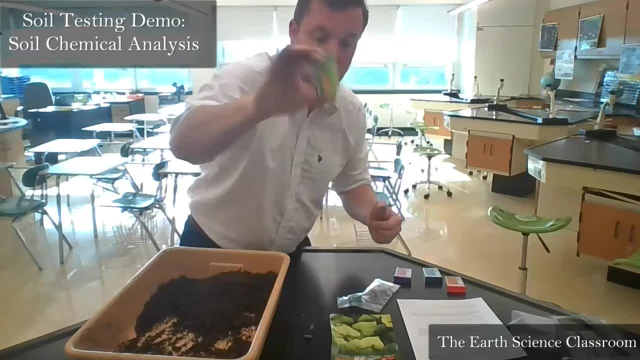 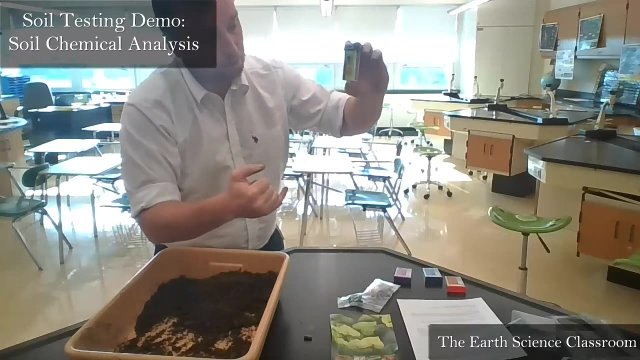 and we shake. we shake for 30 seconds again so we can mix the soil and the chemical indicator and the water. what's going to happen is the chemical indicator once we let go- okay, we stop shaking it- it will start to settle and we have this scale over here. 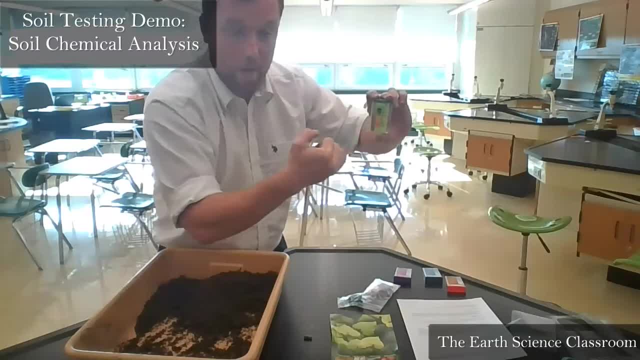 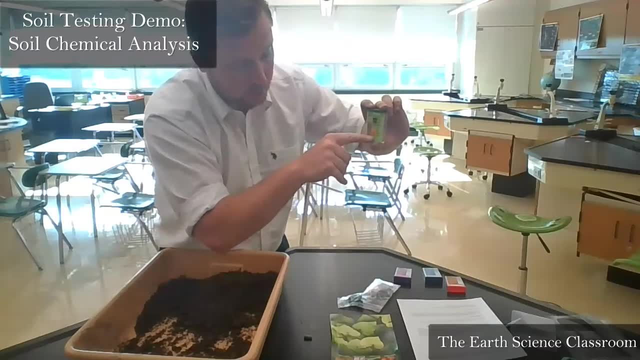 it's a ph scale gives you these colors and that represents the amount of acidity or alkali in the soil. now the lowest one, the red one right here, is very acid or very acidic: ph 4.5- and it goes up so the number increases. so ph 7 is neutral. it's not an acid or base. and if you get to 7.5, this 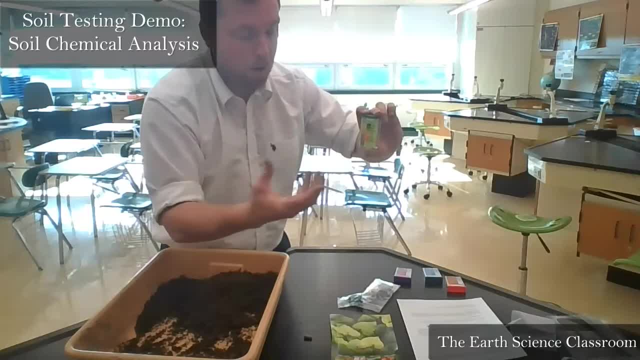 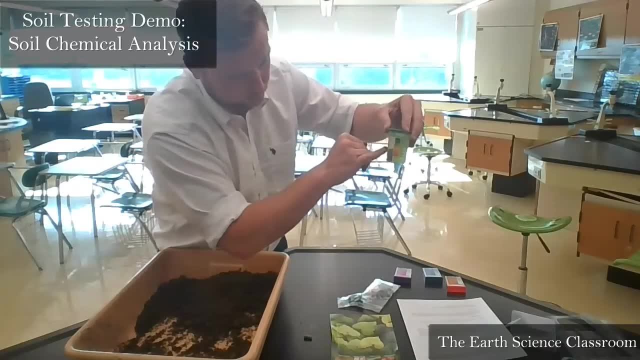 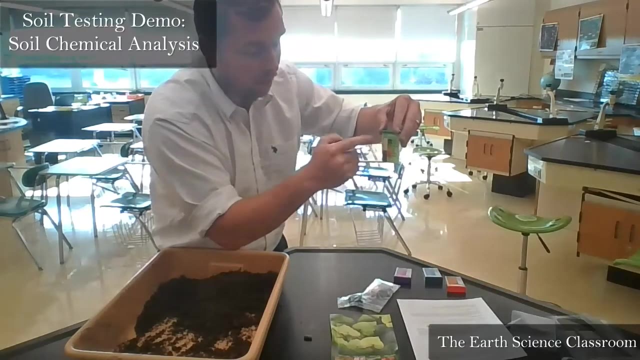 dark green one at the top here is 7.5. that is more of an alkali uh concentration. so the soil will be alkali. what you're looking for is the water. the water will turn a certain color and you match the color of the water with the color of the scale and then you write down. so leave it nice and there. 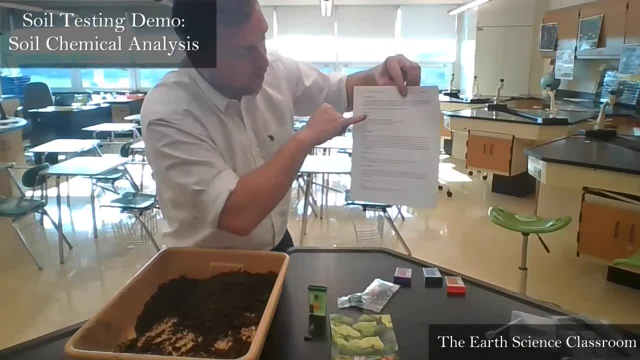 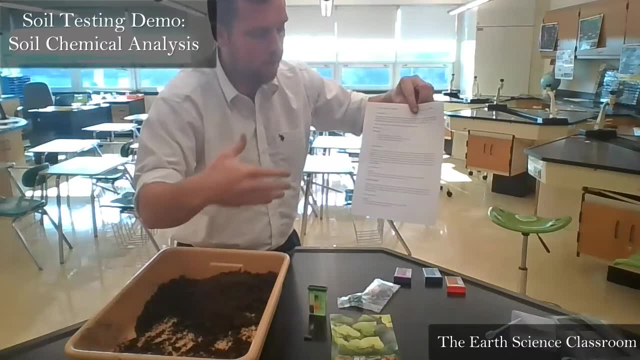 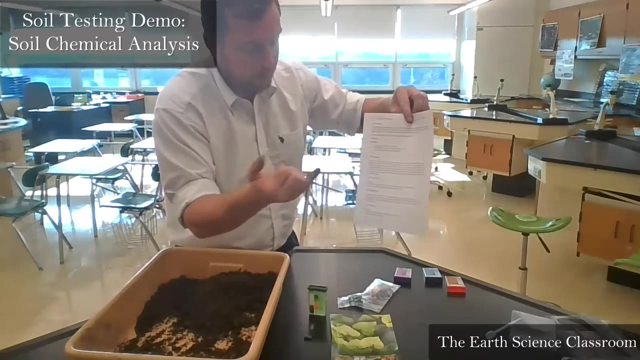 you have your lab and then you write down the ph number: 6.5, 5.55, whatever the color of the water is, you match with the scale and you put the number right there. so let's say our soil is ph 5.5 put. 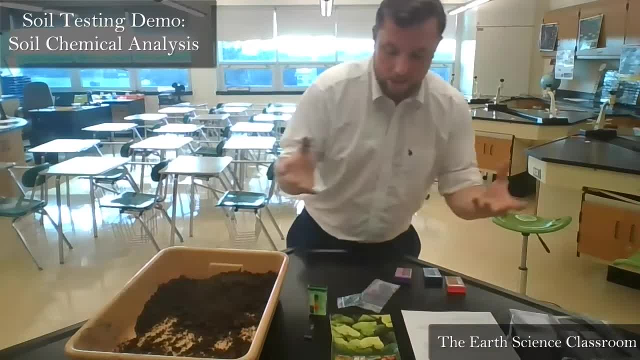 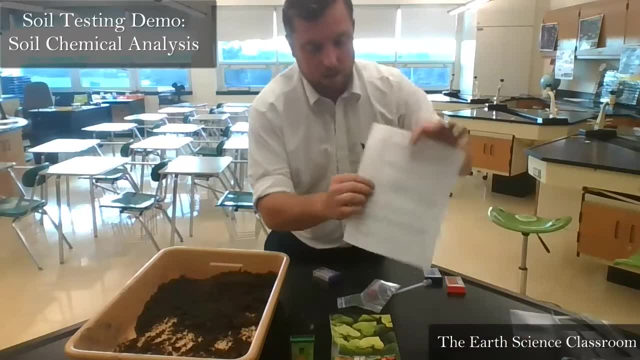 that down and you're done. that's our ph uh test. you leave that there. we take our next one, which is nitrogen, and on the sheets. i'm sure you've got this one right, but chris N Gauss has passed on and it gives you a little. 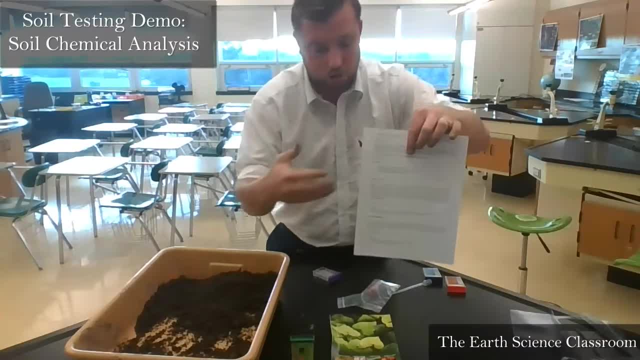 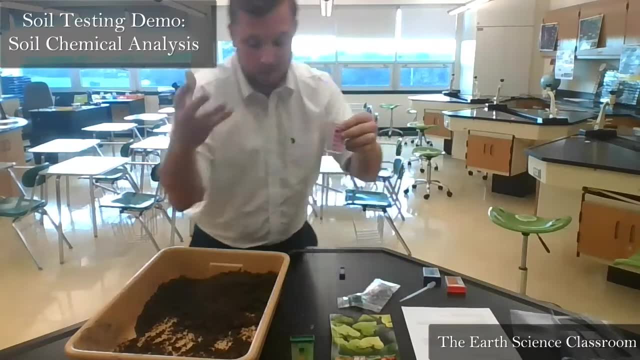 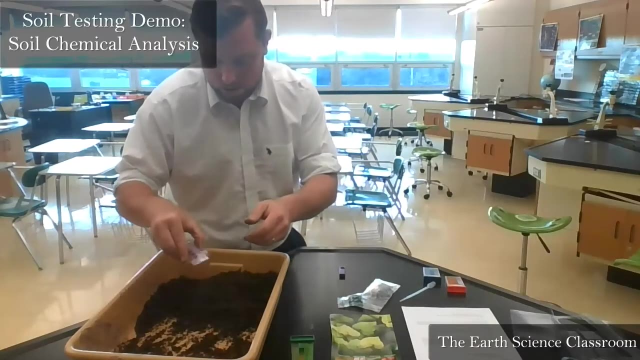 paragraph of why nitrogen is important. what's the why is it there? what does it do, what's its function? so you can read that, if you want to, before your analysis: nitrogen again, do the same thing, repeat the same steps. we get a little bit of soil, but in a small uh compartment. okay. 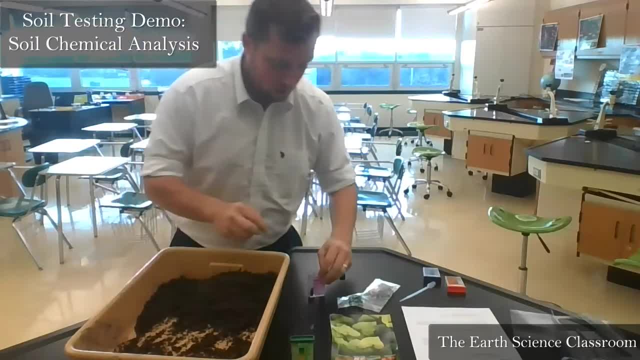 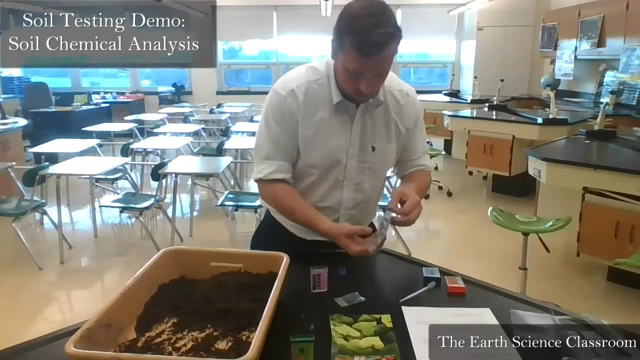 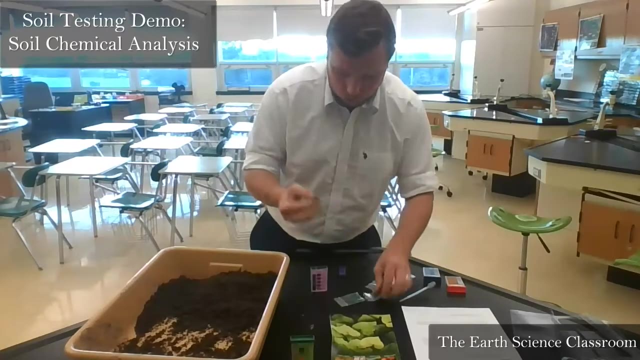 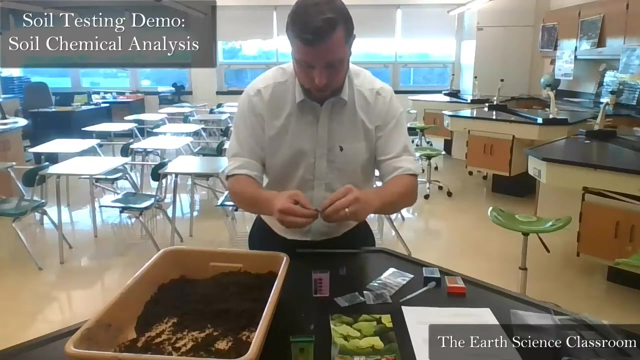 a bit too much. there we go like that: okay, a little bit so, like that purple. So we get the purple chemical indicator in our lab like so: Take one out, One capsule, one indicator per testing time, okay. So we again twist, We twist and release the chemical. 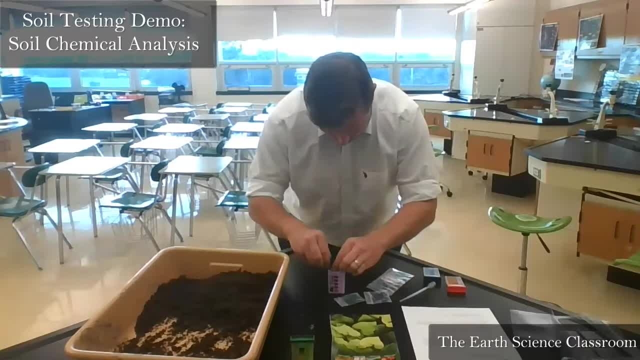 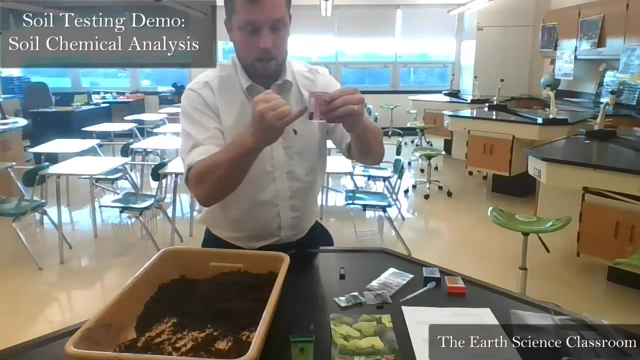 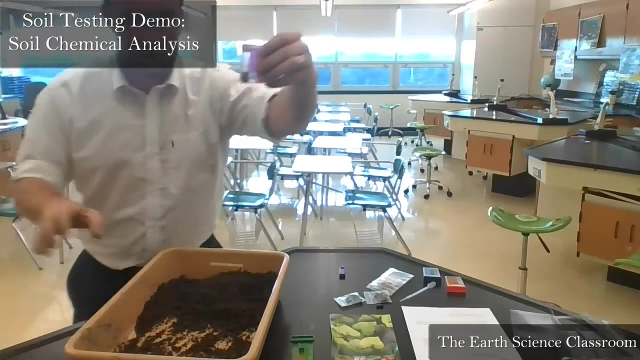 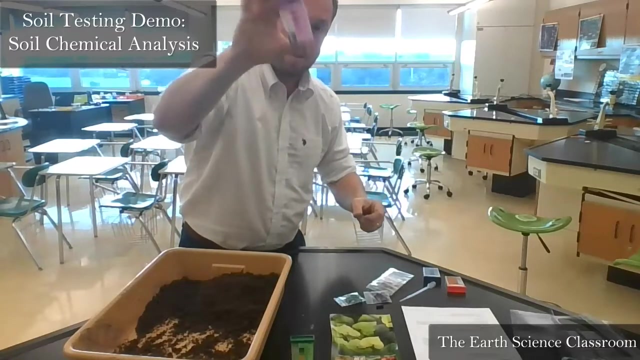 indicator. It'll give us our data, our reading. okay, We have our soil and our indicator And we add some water, like so, All right, And then we put back on the lid, Make sure it's nice and tight Finger and thumb, And we shake to mix the water with the soil and 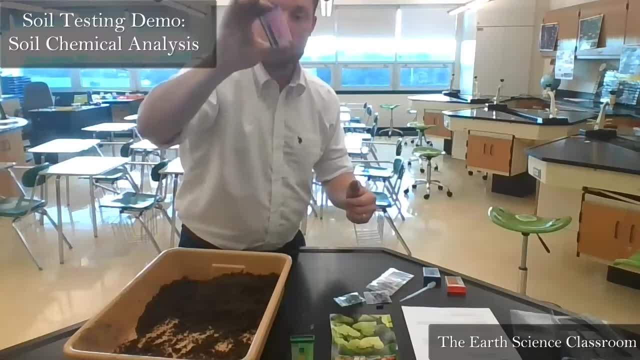 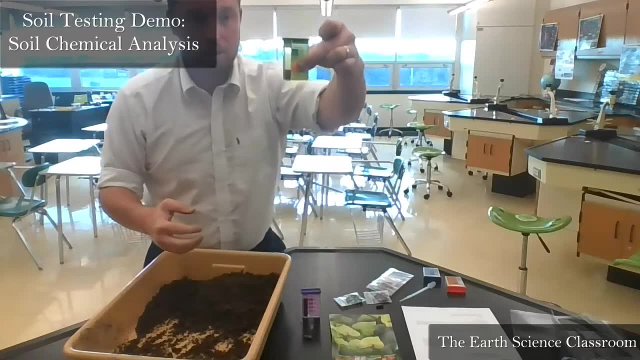 the chemical indicator About 15, 20 seconds. Let it settle. Now we go back to our pH. Look at our pH. Look at that. Oh yeah, So we have this nice color green. right now It's lime green And I would 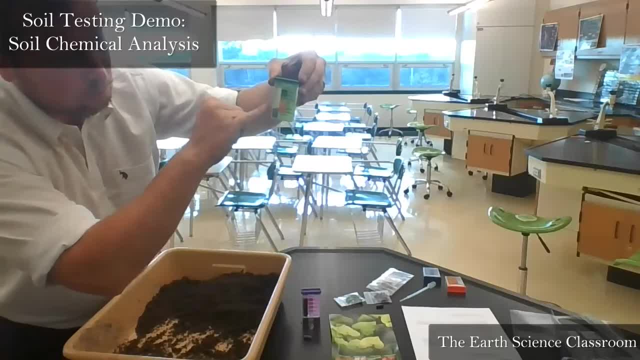 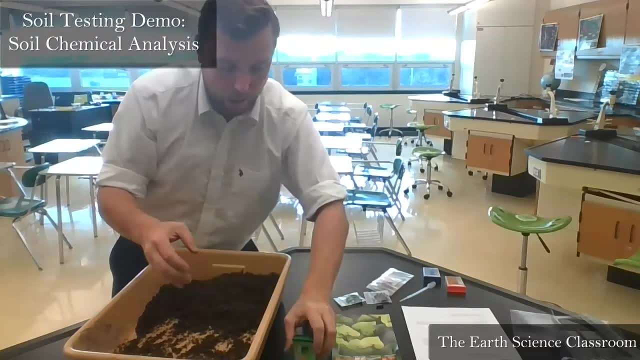 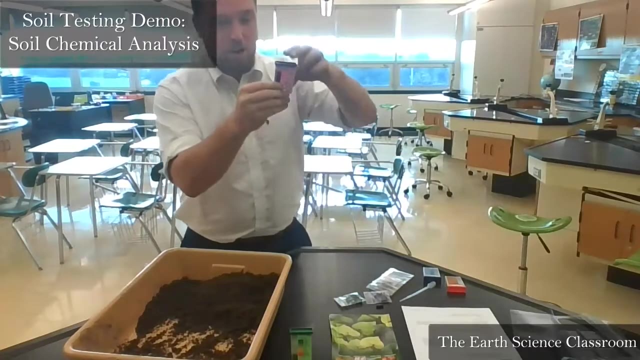 say that would be between 6 and 6.5 on our scale. So I put them on my pH. I would put in 6.5 or 6.25 in between. Again, the color doesn't-. We have our nitrogen. It takes more time to settle, But you should see a change in color. 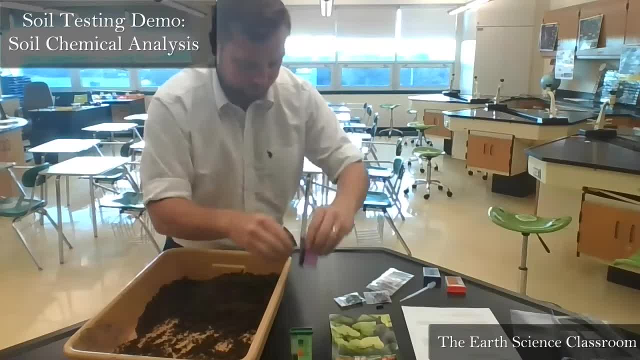 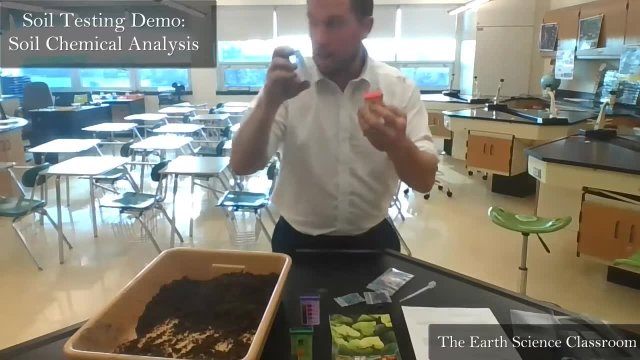 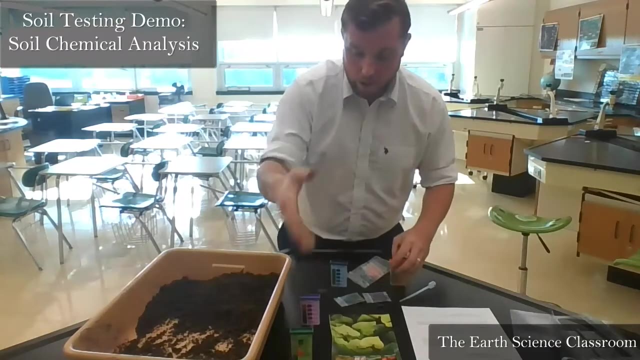 and match it to the amount right here. So, guys, Okay, Two more to do. You have phosphorus and you have potassium. Again, this is the blue capsules and the red capsule- with the same procedure as with the other two, the previous two, and you write down your results.